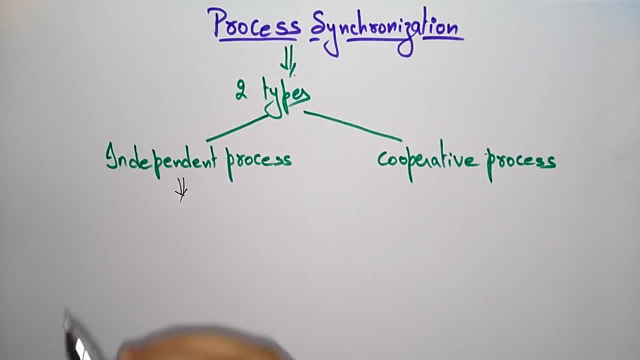 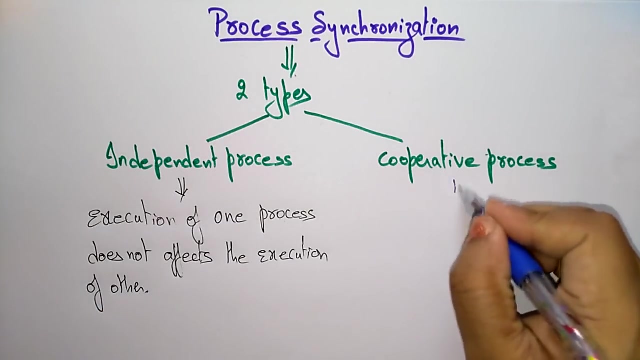 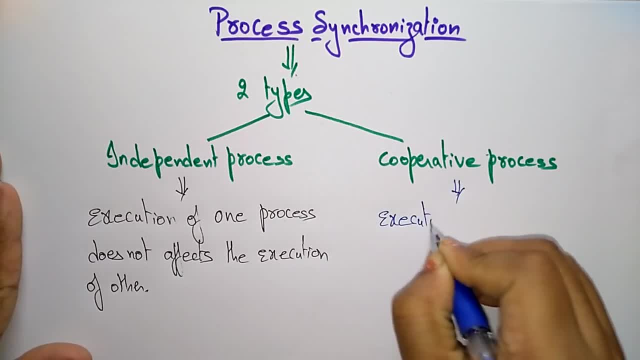 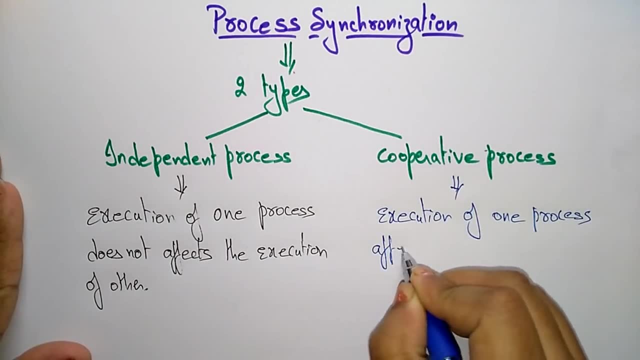 affecting Execution of one process affects the execution of other process, Other process. So that is the difference between the independent and cooperative. The main thing here. you have to be know that it does not affect the executions and it should affect the process, the execution, the process. synchronization arises in the case of only cooperative process. 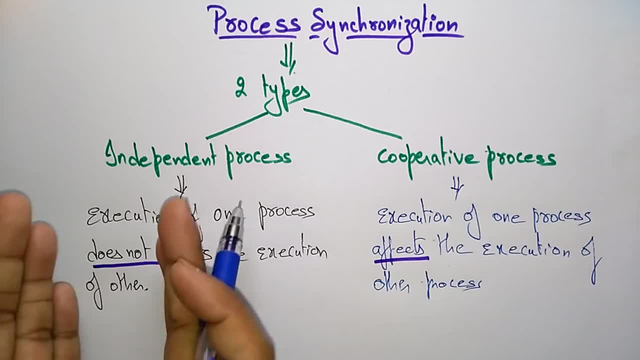 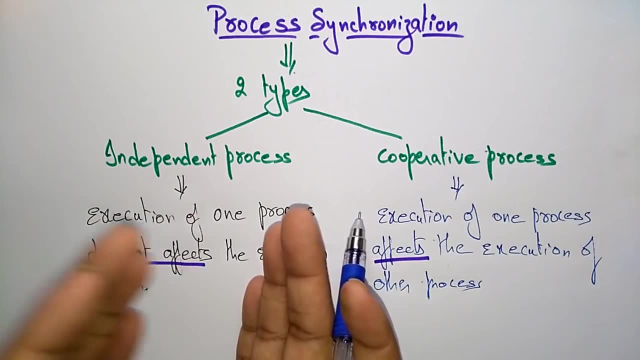 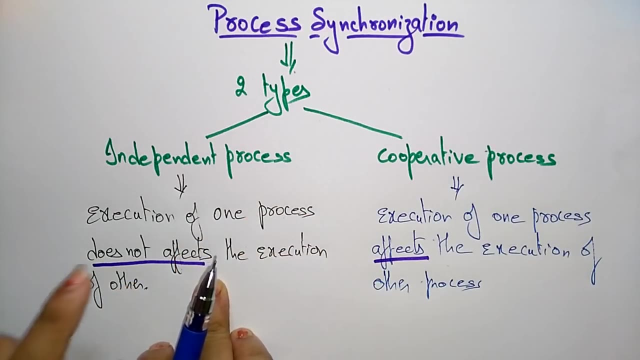 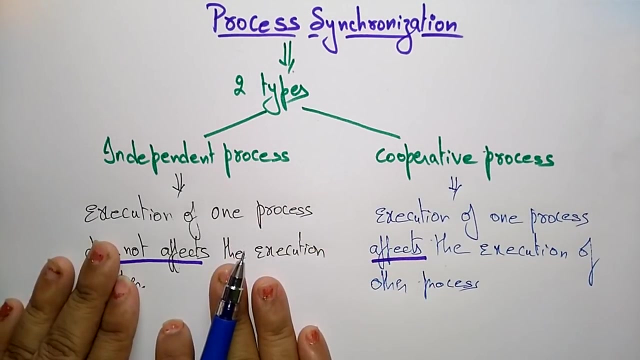 why it is arises only in the cooperative process. so if you take independent process, there is no dependency relationship between one and another process. so here a synchronization problem will doesn't arises. okay, because each process is independent. they are not sharing the resources. each process is having their own resources, okay. so that's why there is no problem here in. 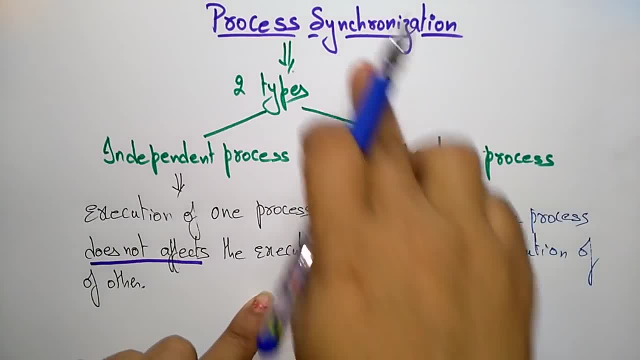 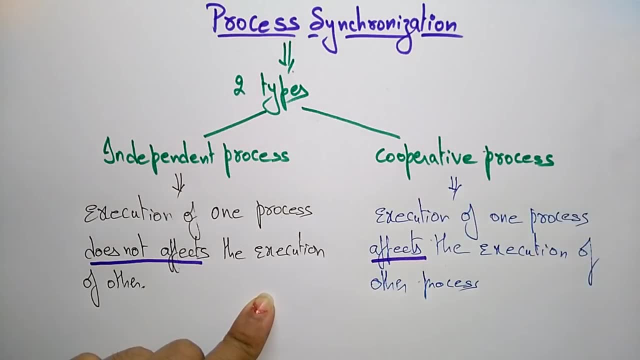 independent process, whereas in cooperative process the process synchronization arises in only the cooperative process. so also because resources are shared in cooperative process. so let me take one simple example: it's alive. suppose if you are all the people, or suppose a committee is there. so every, every, every. 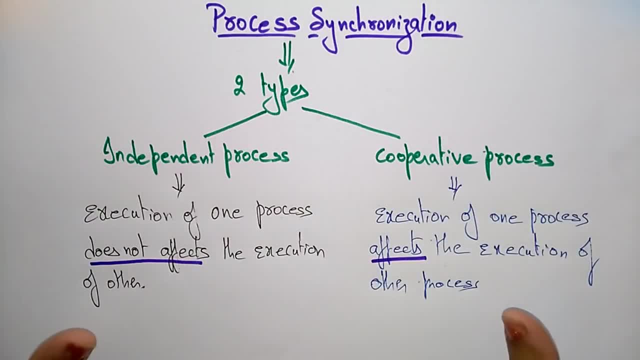 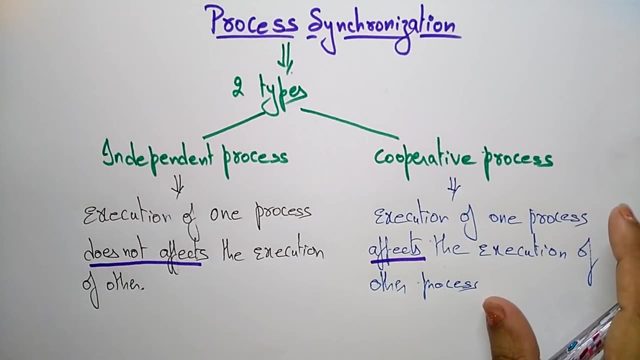 everyone was watching us one movie in the community hall. okay, so in the amphitheater. so if you are watching the same movie, means in your homes it is independent, means whatever you want you can watch, but while you are watching the one movie along with all the people there, 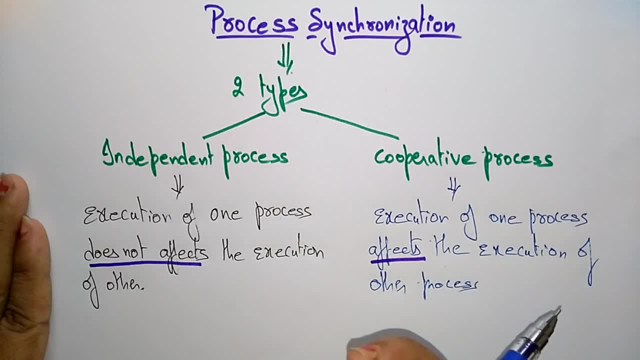 should be a cooperation between those people, because you are using the same resources. so one movie was watching everyone. so there should be some synchronization between the each one means after this movie we will watch another movie, after that we will watch another movie. like that there is a cooperation should be there. so the execution of one process obviously affects the execution of 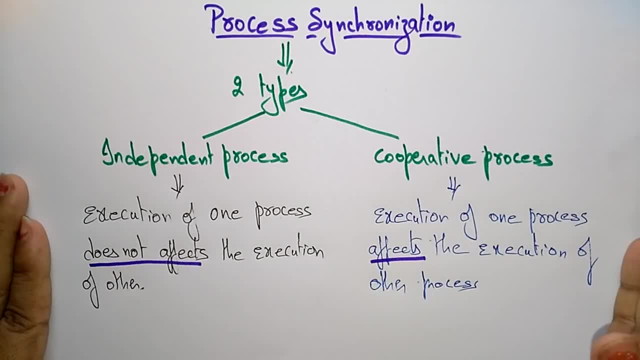 other, because one person may interested one movie and another person may interested in another movie he wants to see. he don't want to see that movie. so there the process synchronization problem will rises if you are watching the movies in at your home, not stay alone. okay, so then there is no problem for you because you are having your own resources. 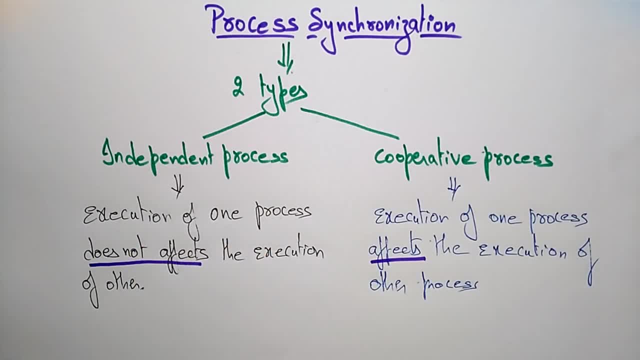 your own TV. so that is a general example. I am saying that the process synchronization. so whenever there is an independent processes there is no problem in process synchronization. so the main process synchronization arises only in the case of cooperative process, also because the resources are shared in cooperative process. so let me explain a critical section problem. 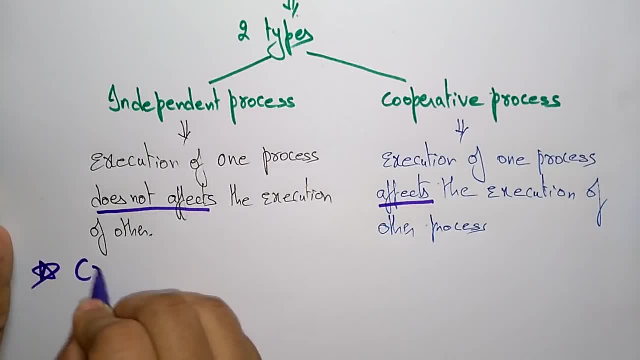 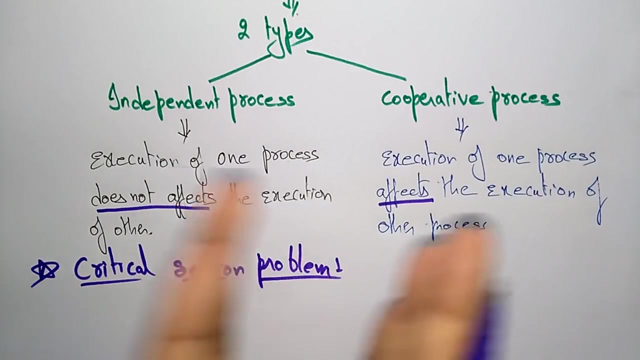 critical section problem. so you may get doubt. what is it critical section problem? so I didn't explain about critical section, but I'm explaining about the critical section problem. so what did it mean exactly? so you understand what is an independent processor and what is a cooperative process so critical. 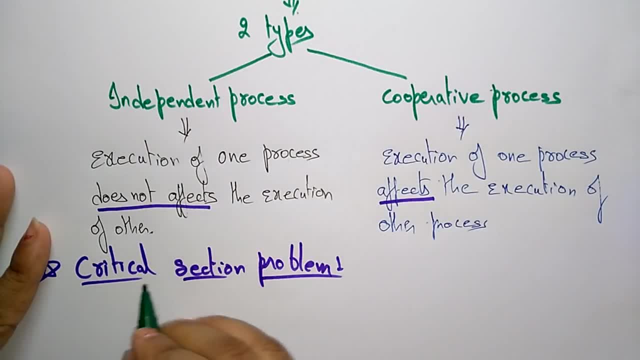 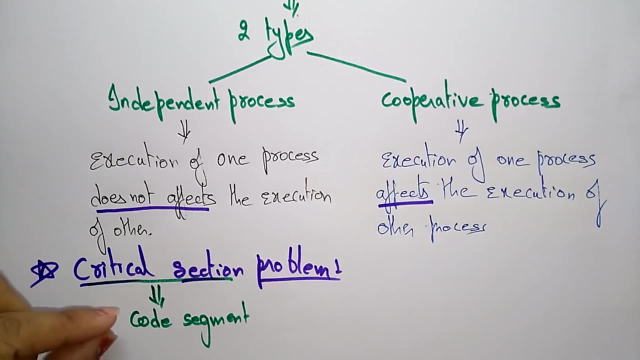 section means actually it is nothing, but it is a code segment. A critical section is nothing, but it is a code segment. So this code segment that can be accessed by only one process at a time, So only one process can execute that critical section at a time- It contains shared variables which need to be 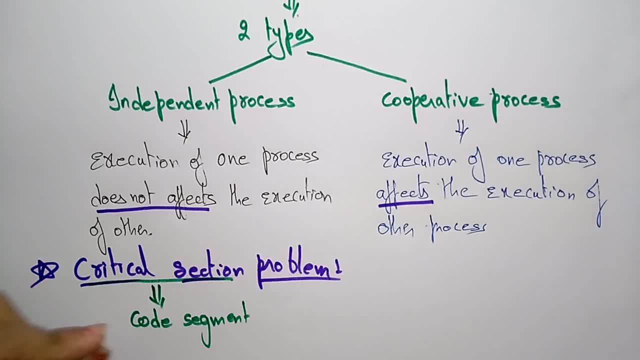 synchronized to maintain consistence of data variables. So the critical section is all, it is nothing. but it is a code variable. So code segment, it contains the shared. shared variables means everyone can use. means suppose if you take that whatever amphitheater I had explained, So they that movies have to be wash everyone. that is a shared variables. 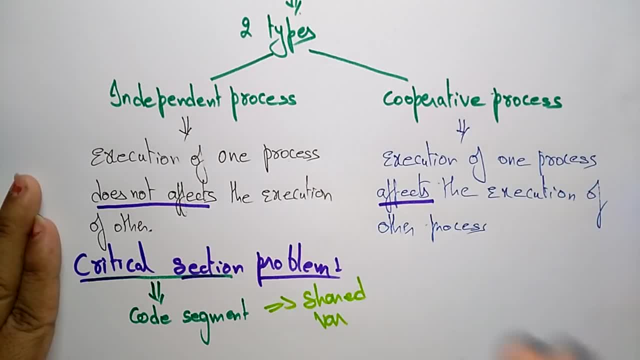 So if suppose, if you want to solve the problem of process synchronization, or you can say, if you want to solve the critical section problem. So I said, critical section is a code segment. So if you want to solve the problem of process synchronization, or you can say, if you 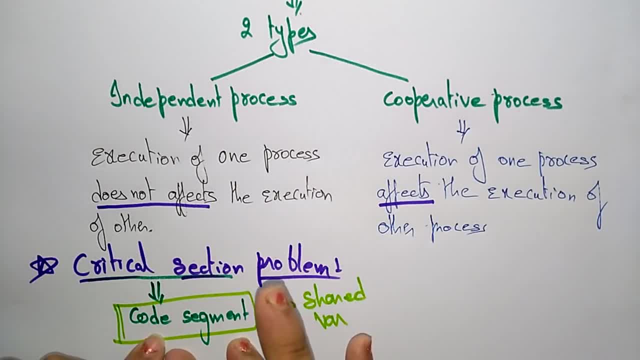 segment. So means it is a movie that we want to watch. So this movie is using the shared variables. means amphitheater. we are using shared variables, Suppose, if a group of team- that P1 process- is consisting of a group of team and P2 is another group of team, P3 is another group of. 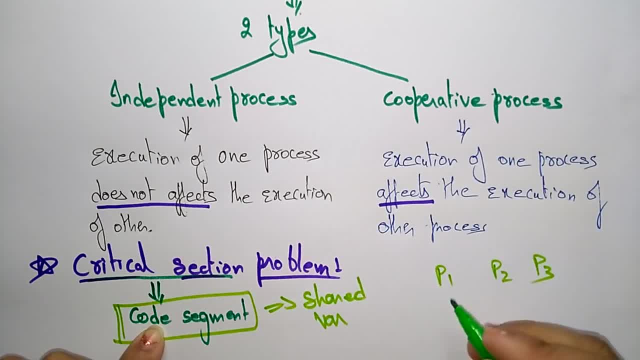 team. They are come to an understanding: P1 wants to see the movie A and the P2 wants to see the movie B and the P3 people wants to see the movie C. So everyone will use the amphitheater. that is a shared variables. Okay, A, B, C, this all movies. 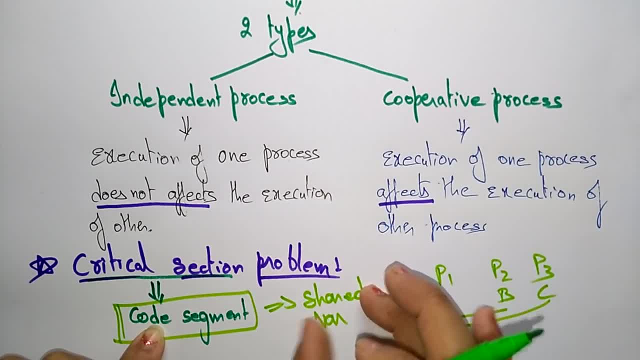 has to play in only shared variable, that is, amphitheater. So then the critical section: what it does the people who wants to see the A movie first, they will be freezed, They will reserve the amphitheater. So whenever they reserve the amphitheater that you call it as a code segment, 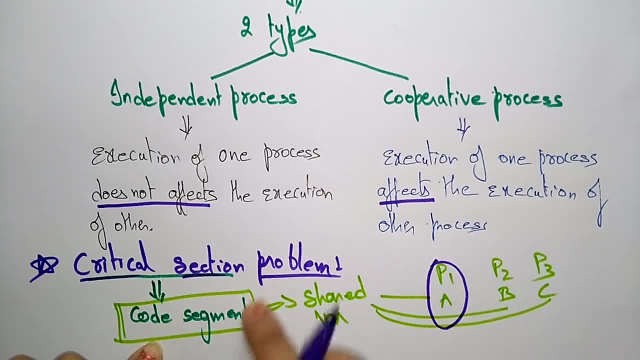 They are executing, critical section is executing. So whenever this critical section is executing, the remaining people has to wait until the chance will come. Okay, So next and the person will come and they will watch. next and the person will come, they will watch. Okay, So this is a mutual understanding between these problems. So this: 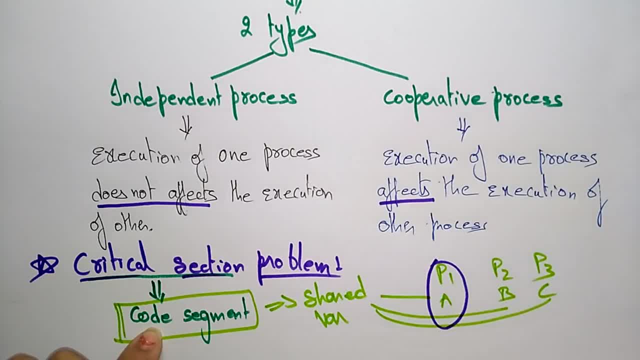 critical section problem can be solved by using some different solutions. So actually critical section is just a simple code segment. So if you want to execute that movie, if you want to see that movie, that is a A, B, C movie, Okay. So if all the people 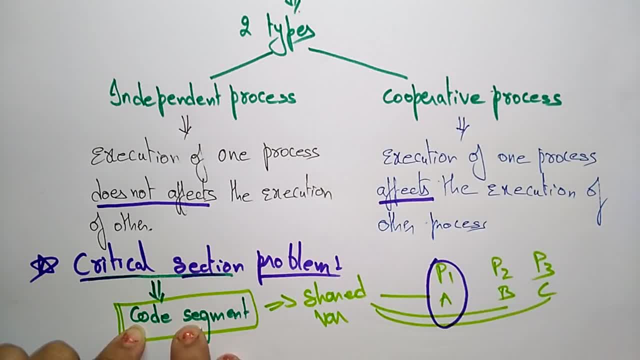 wants to use the shared variables, So there is a problem arises. So that problem- you call it as a critical section problem, So that can be solved by using this one technique. This is a shared variable, means the shared variables are accessing by each person with mutual understanding. So okay, 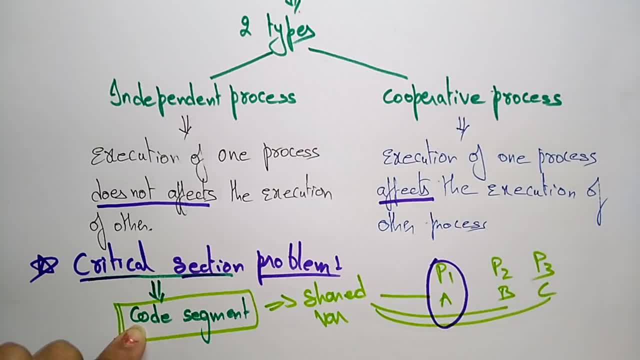 first you watch and second you watch and the third you watch, like that. Okay, I hope you understand exactly what the critical section, So don't be confused. Critical section is nothing but a code segment. Okay, That code segment want to be executed by all the 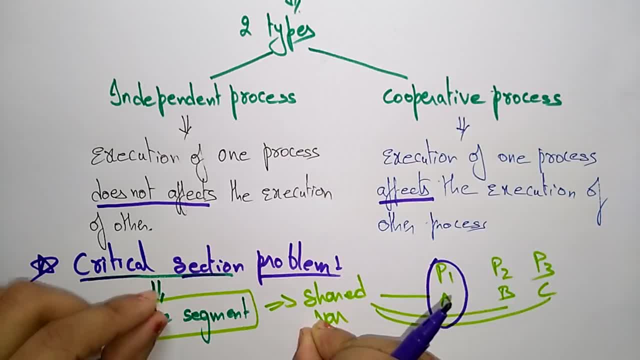 processor, Okay, By using the shared variables. So if all the processor come at a time, by using the shared variables, Okay. There is a problem arises. Suppose this person wants to see the move at that time only and then the person also wants to see that movie at the same time. means 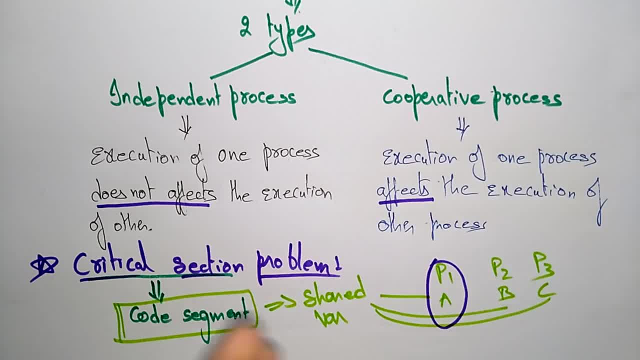 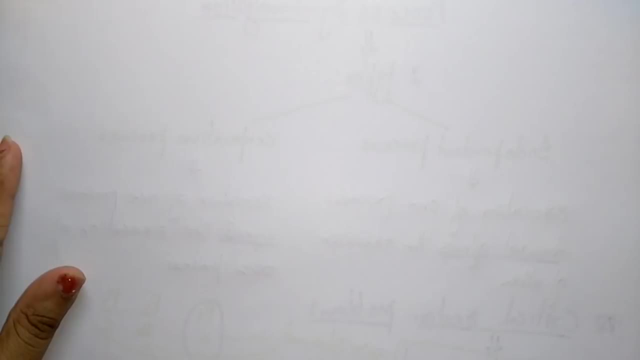 some disturbance will occur. Okay, That affects the execution of the processor. That movie will not be played at that date. So that is a problem. That is a critical section problem. So I will just write the sample code for this critical section. So actually the critical section is a code segment. 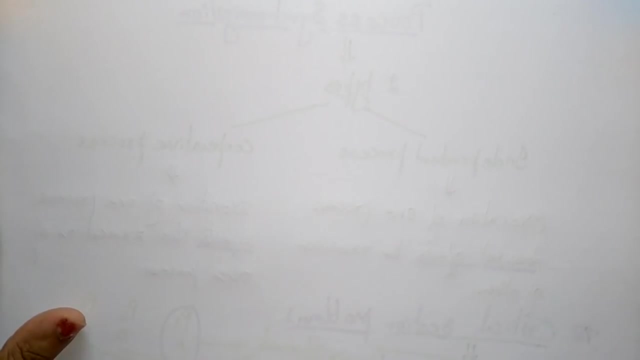 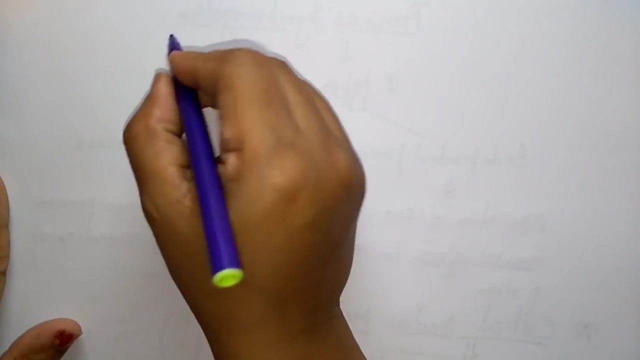 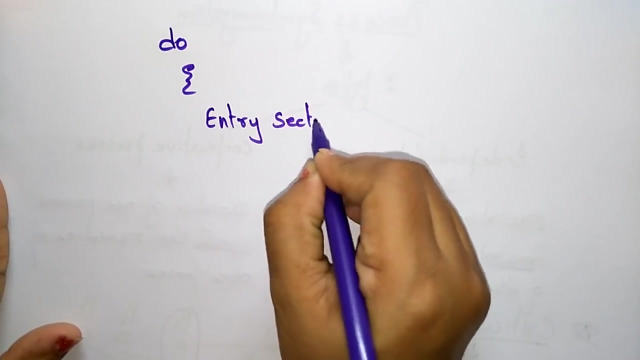 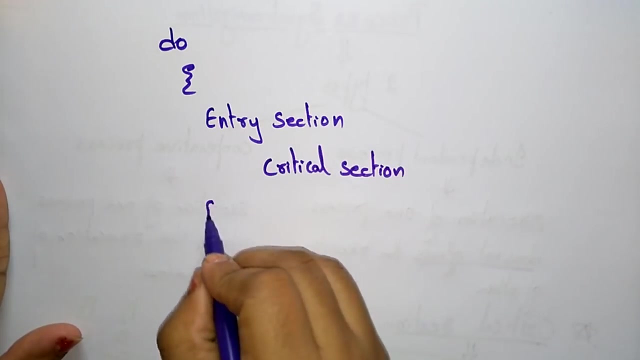 that can be accessed by only one process at a time. It contains a shared variables which need to be synchronized to maintain consistency Of a data variables. So do. This is the entry section. Next, critical section. Next, exit section. Next, remaining remainder section. 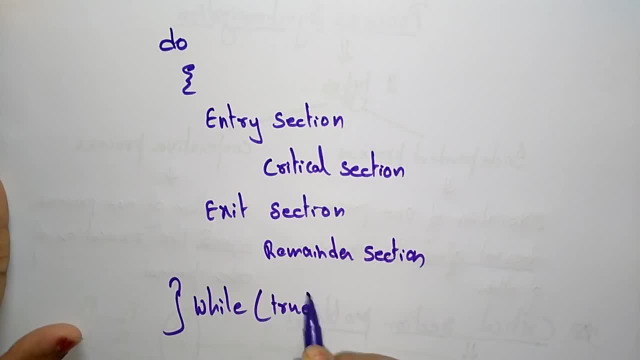 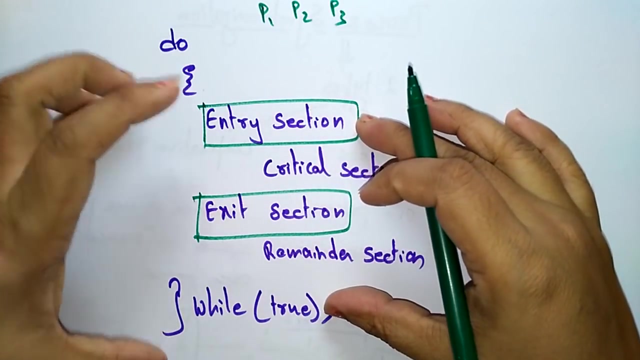 While, While this is true, Then it will execute this process. So here they are saying that this is an entry section and exit section. So once one process- Suppose P1, P2, P3 process- wants to use this, the same resources shared. 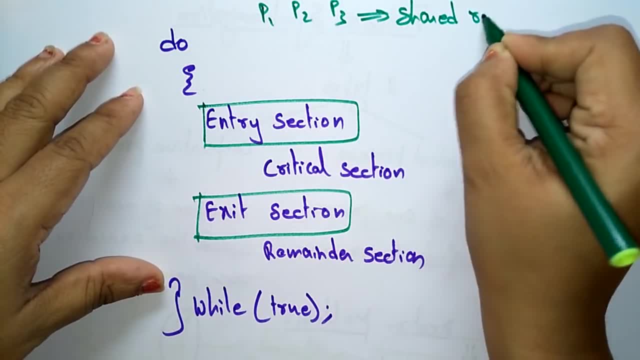 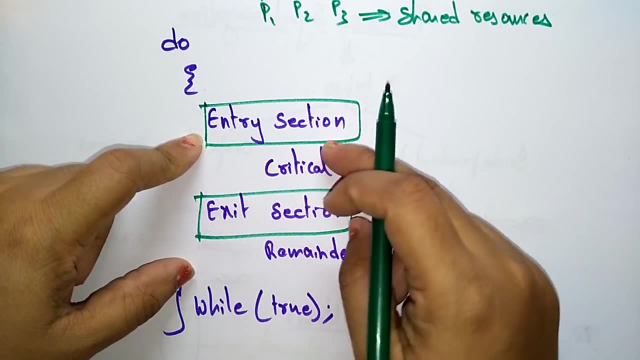 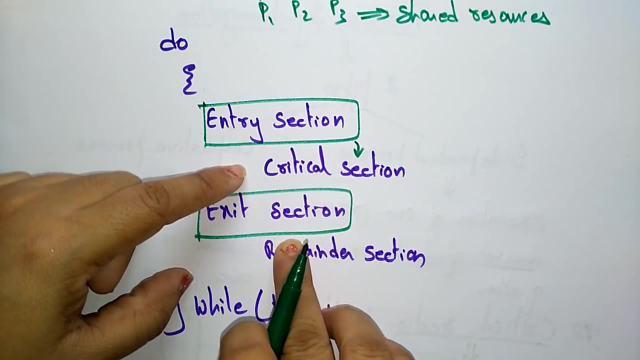 resources. They want to use the shared resources. So when they want to use the shared resources, First the P1 will enter the entry section. So whenever it entered the entry section it satisfies the condition, It goes to the critical section section. so so until it enters the exit section, no other process will enter into. 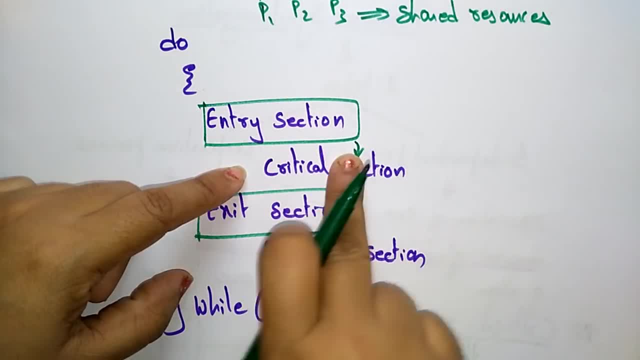 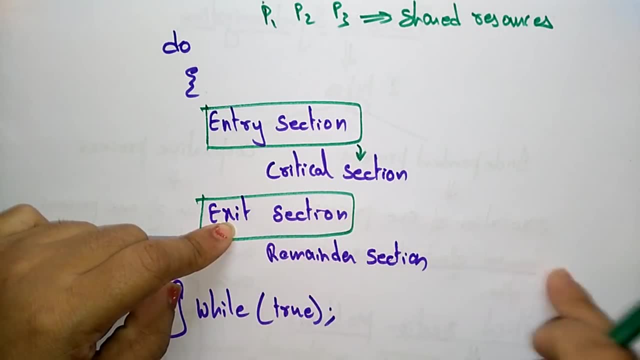 this critical section. okay, suppose P1 work is over it, he watches the movie. okay, then it intimates with the exit section after exit section. it will do its remaining remainder section means it doesn't affect the. this remainder is independent. so this and the process will continue with the remainder section. so 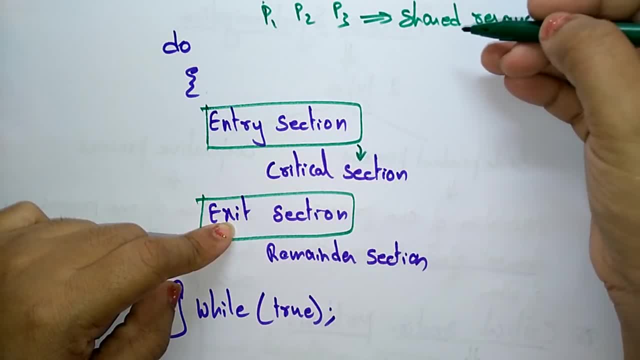 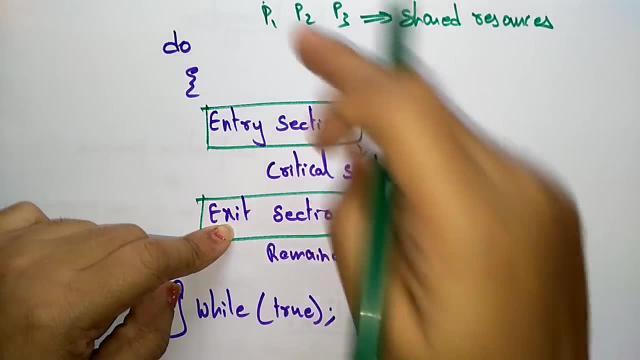 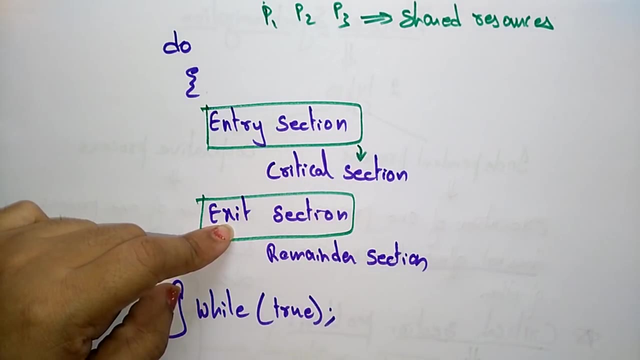 only the shared resources which are using the shared variables. they can use only entry section and exit section and that program will execute in critical section. and if the this P2 don't want to use the shared variables, so P2 directly enter into remainder section and execute the program. so each process. 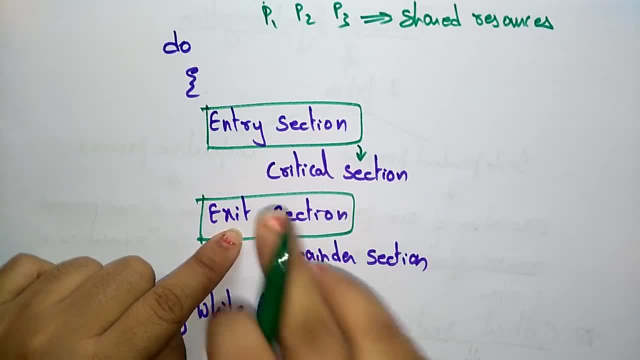 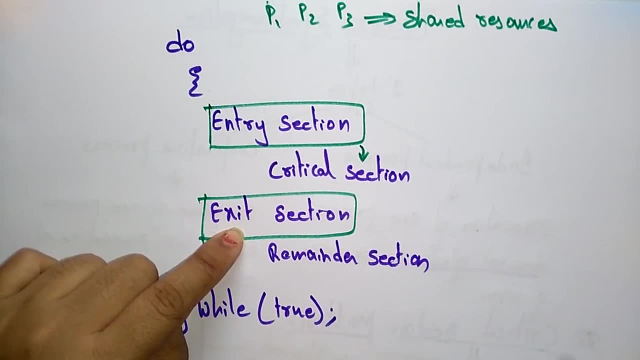 when they want to exit they have to enter the exit section. these exit section will intimate to other process that okay, critical section is free. you just enter into critical section. you can use a means: removes the lock. entry section will make the lock and exit section will removes the lock. 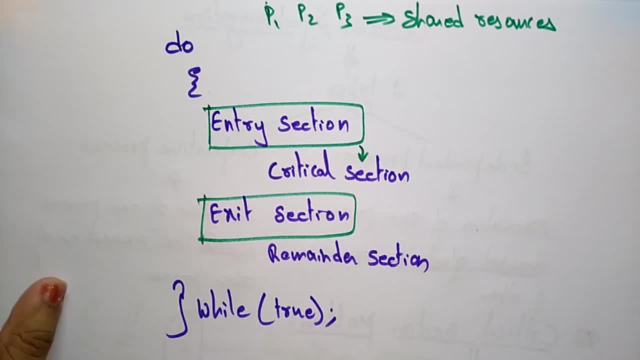 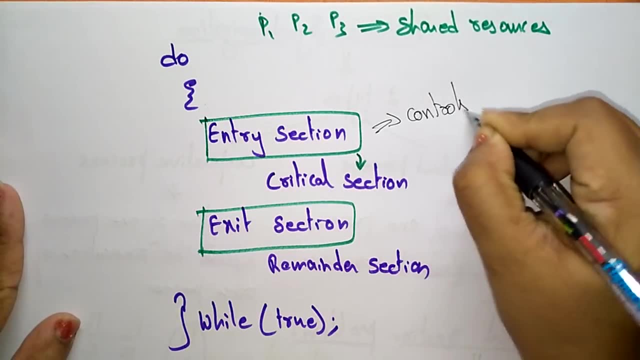 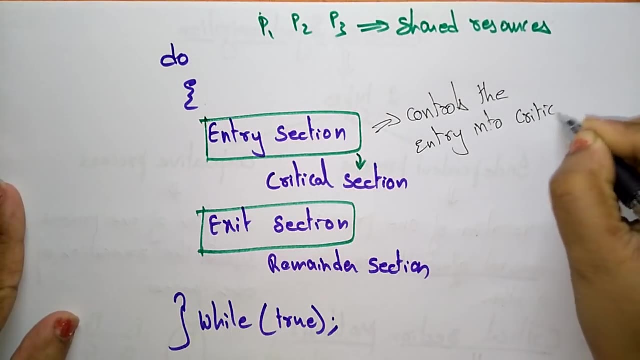 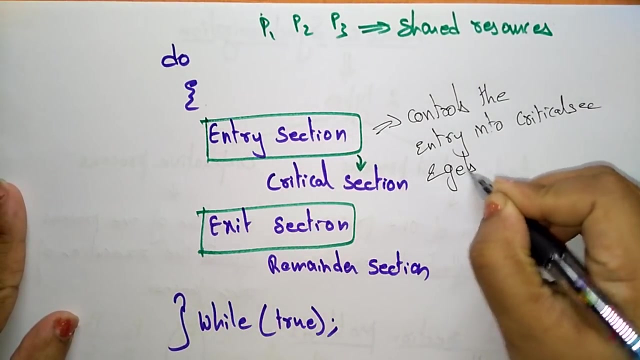 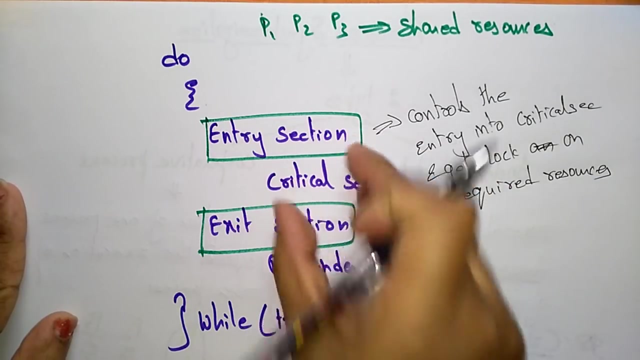 ok, so let me write that point, then you'll understand. entry section controls controls the entry into critical section. entry section controls the entry into critical section and gets lock. gets lock on required resources. so whatever the resources that process is using- that is a shared resources- that will be locked and it will continue in the program code execution, so critical. 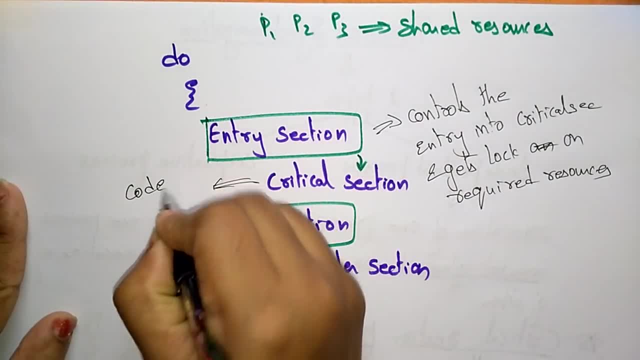 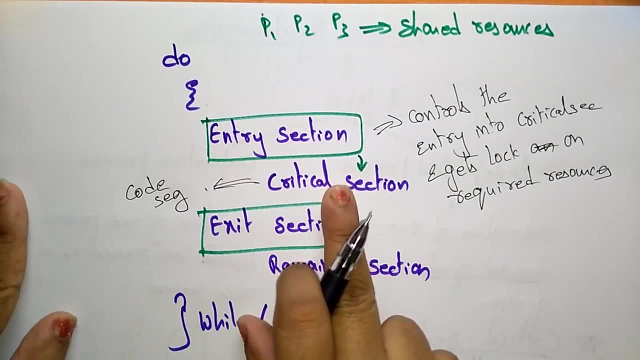 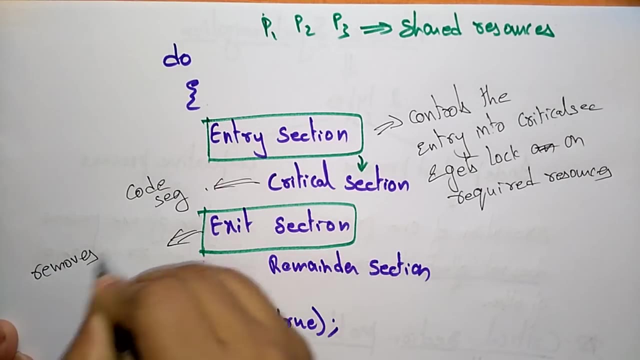 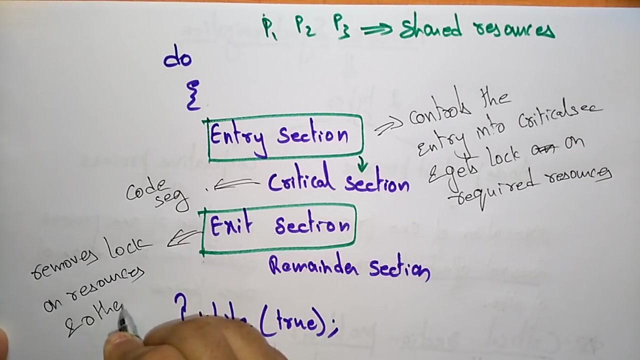 section is nothing but a code, code, code segment. by using the shared variables, it is executing in critical section. so So after that process work is over, exit section will. removes the lock. removes lock on resources and others know that its critical section is over. critical section is over. 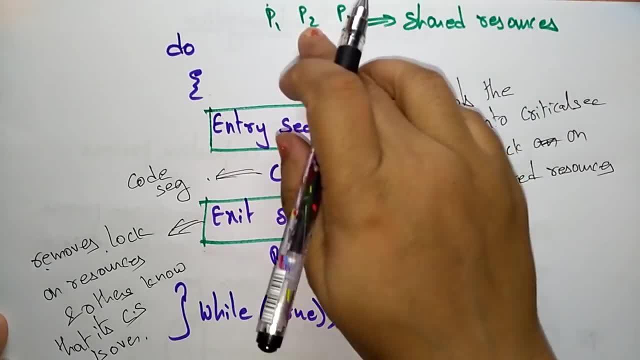 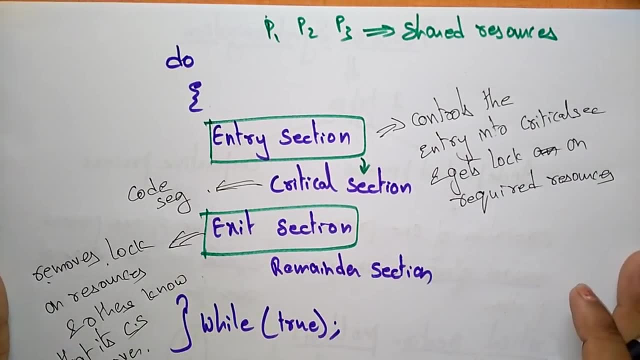 So whenever this lock is removed, so then other process, the P2 will know. okay, the critical section is over, so I can enter into this critical section by using the shared variables. So whatever the process, that using the shared variables, that other process will not use. 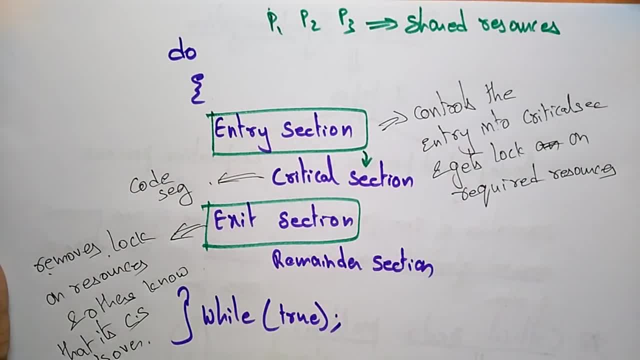 that variables until it exit from the critical section. This is actually the critical section problem. So this critical section problem can be solved okay. So here I am saying: P1 is entering now next, P2 is entering now, next, P3.. 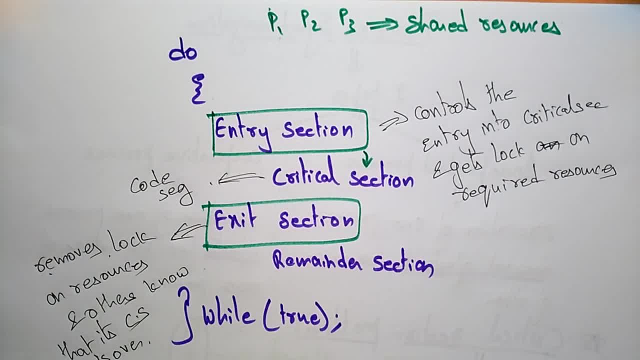 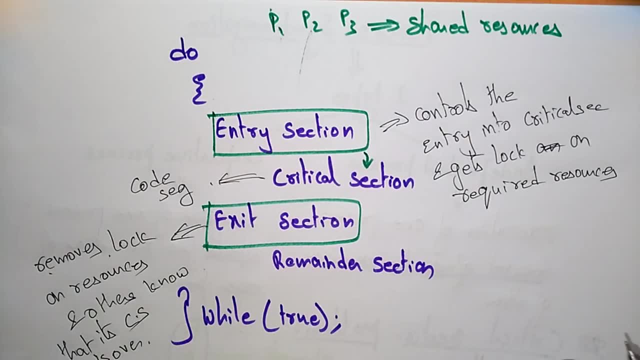 So how can I say those people: those process will enter Okay at a time they will also enter okay. So then the process will not understand which process I have to be taking. So that can be solved by using this critical section. problems can be solved by using some. 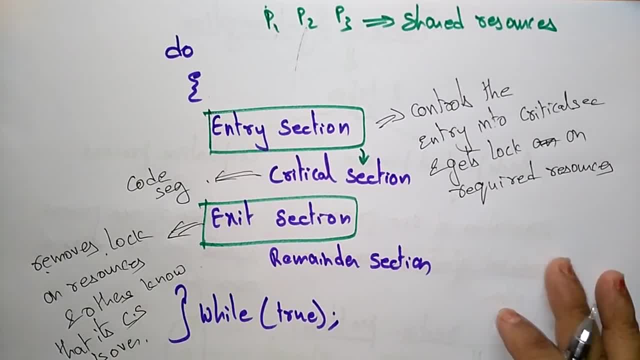 solutions, So that I will explain in the next video. Thank you,